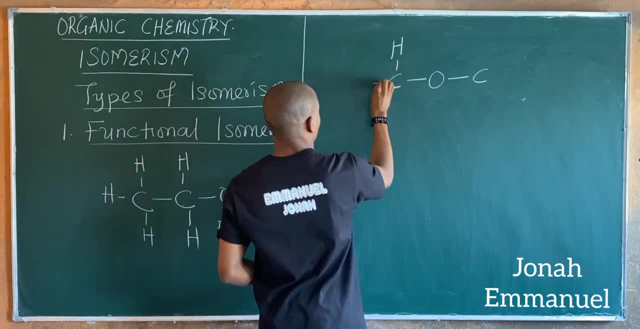 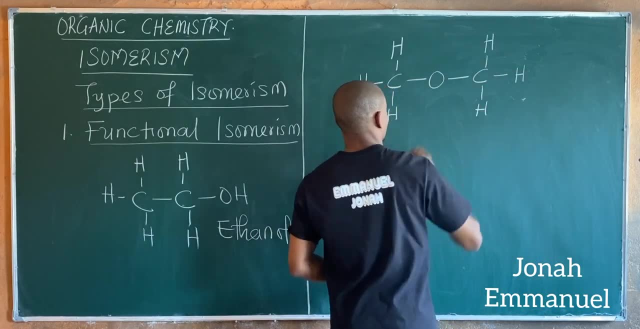 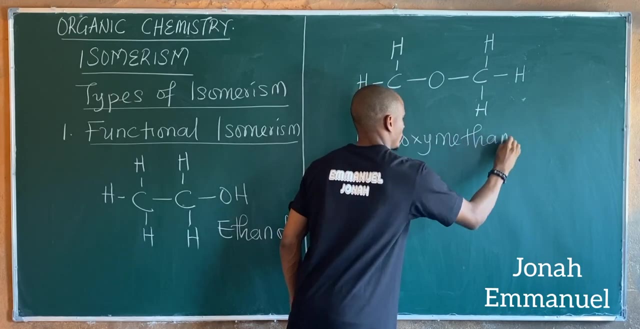 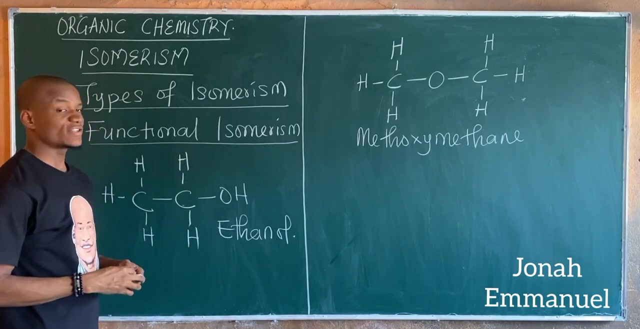 This is the formula for methoxy-methane, Alright, So this is like a methoxy-methane, Alright. two are functional isomers, or they exhibit functional isomerism. Why? Because they have the same molecular formula For ethanol. if I should count the total number of carbon. 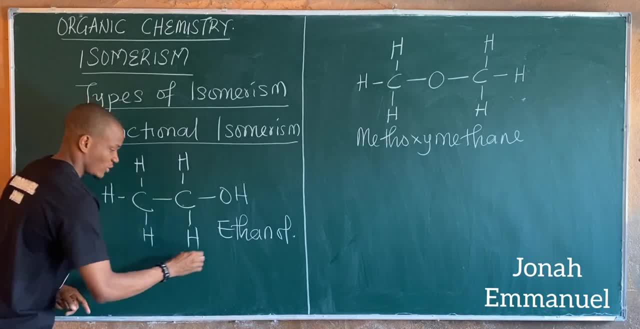 atoms. here for ethanol I have one, two, So carbon is C2, two carbon atoms. If I should count the total number of hydrogen atoms, I have one, two, three, four, five, six, So it gives you H6. And then I have just one, oxygen. So this is like my total molecular 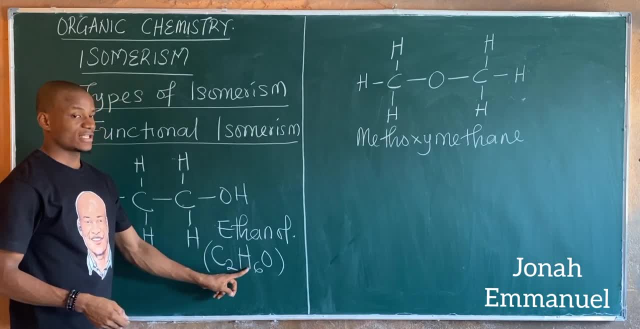 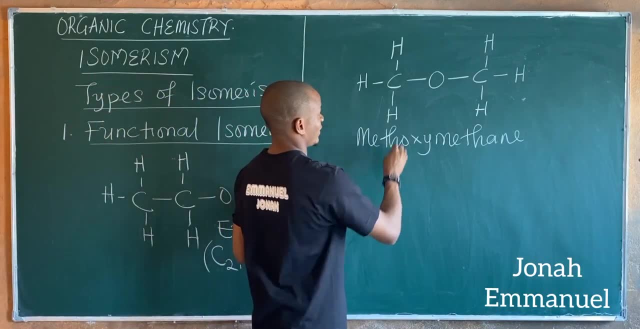 formula For ethanol I have two carbon, six hydrogen and one oxygen For methoxymethane. if I count the total number of carbon I have here, it's one, two, So that's like C2H Count. 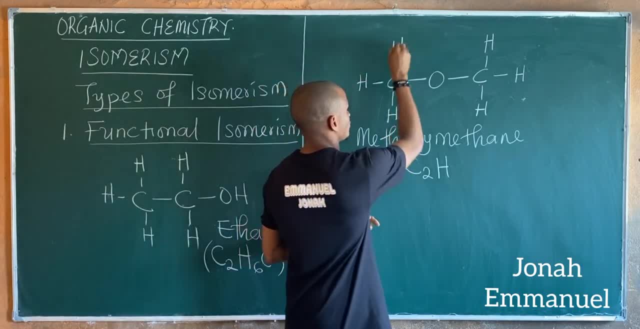 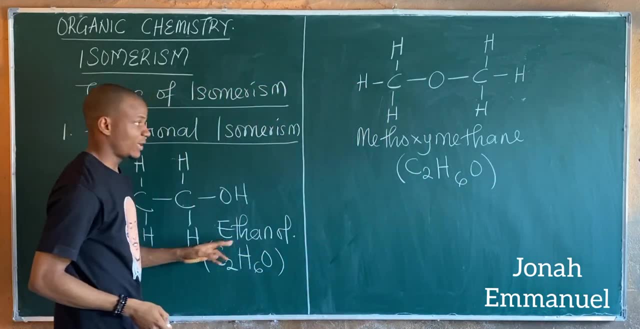 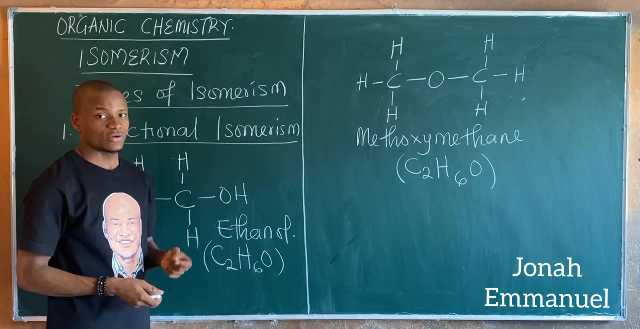 your total number of hydrogen atoms. I'm having one, two, three, four, five, six H6. And then of course one, oxygen. So if you observe, both ethanol and methoxymethane, both have two carbon atoms, six hydrogen atoms and an oxygen atom. So they have the same molecular 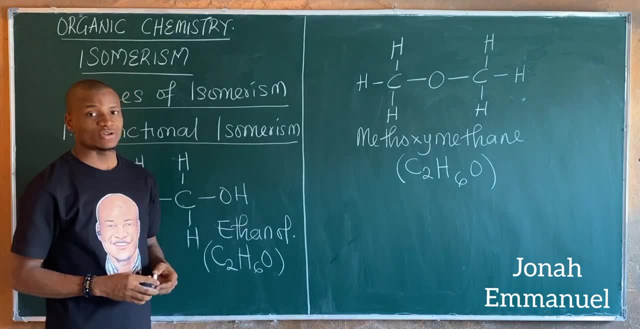 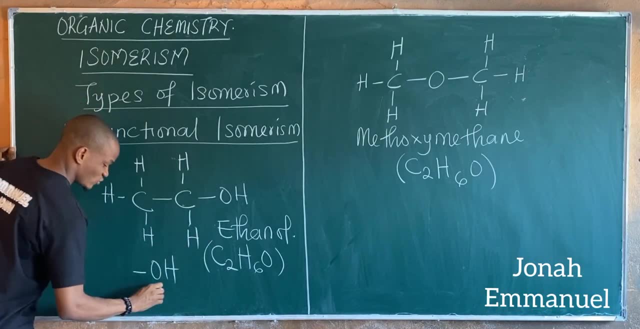 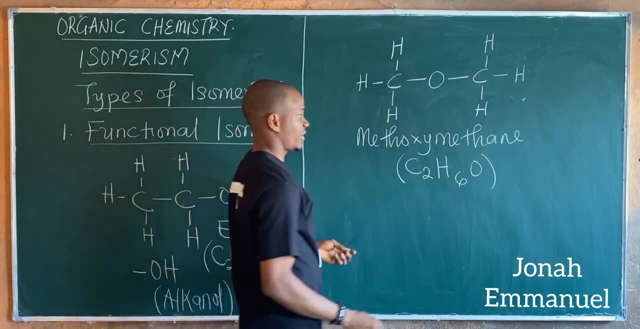 formula Why they are functional isomers? Because they have different functional groups. For instance, for the ethanol, the functional group here is OH, making it to be an ethanol, While for methoxymethane, yeah, the functional group here is OR, making it to be an. 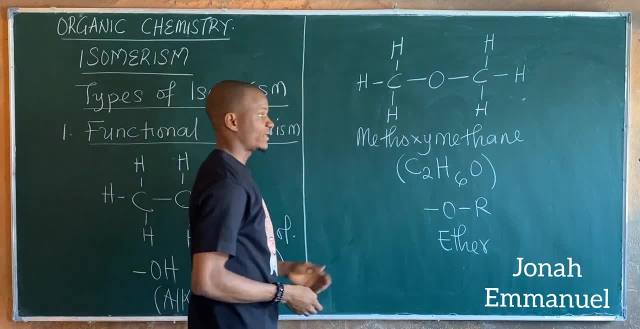 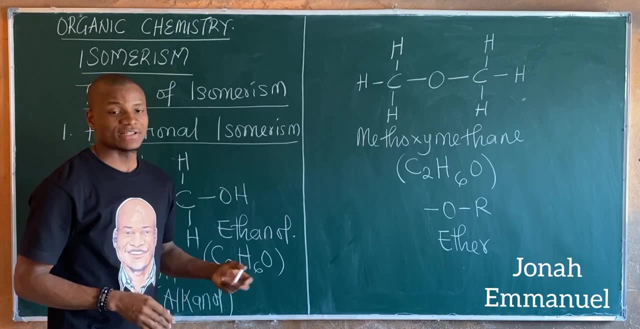 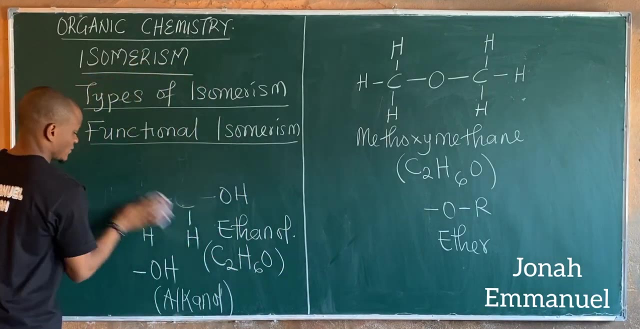 ether. So this is why they are functional isomers. Okay, The same molecular formula but different functional group. So this is the first type of isomericin we have. The second type of isomericin we have is known as chain isomericin, So my number two type of isomericin. 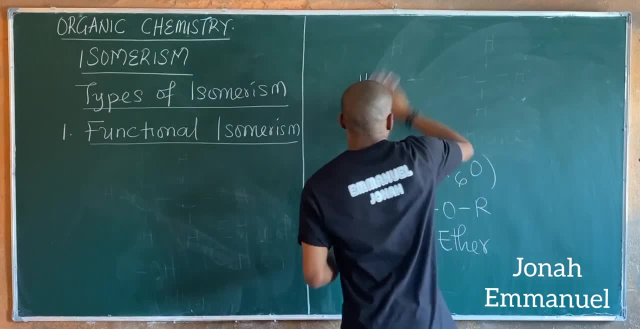 is chain isomericin, the first type, Common. okay, Not use it too many times over With phenotypinamide: Okay, I sometimes do over three times, But with finest creatinine it's called chamomile instead of phenocytinamide. 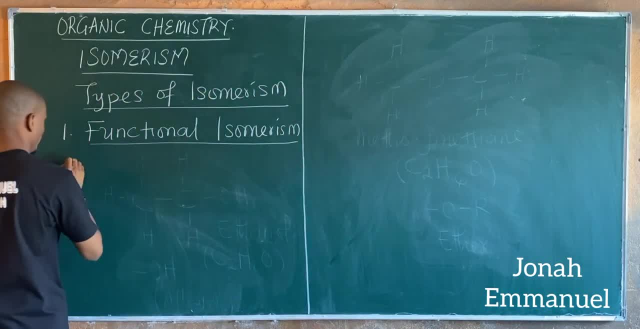 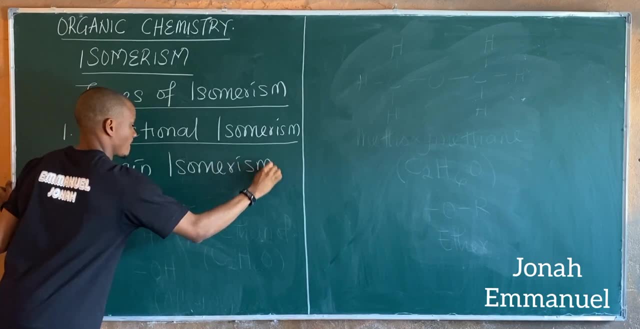 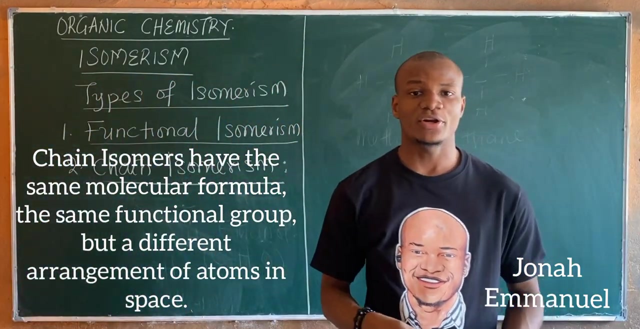 So whatever isoprenicin or denominative for the'veon. But I guess the main reason why these people chain isomerism: Alright For chain isomerism. they have the same molecular formula, They also have the same functional group, but they have 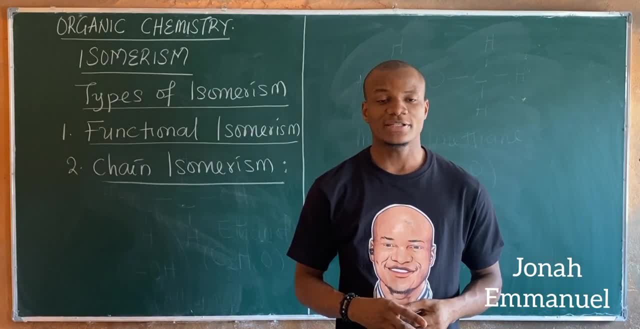 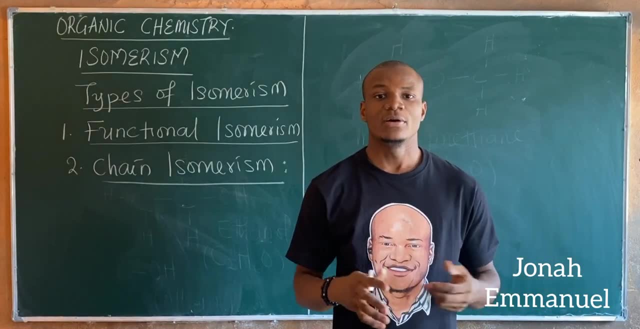 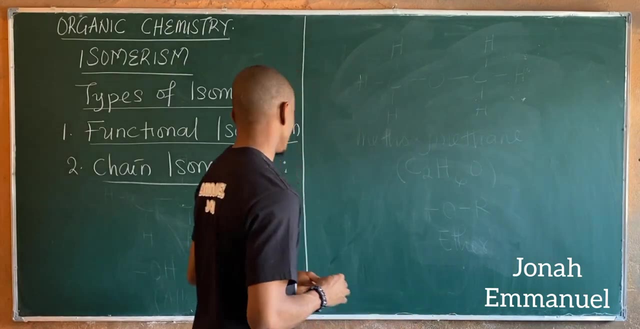 different arrangement of atoms in space, For instance, compounds that exhibit chain isomerism. includes butane and 2-methyl propane. Alright, So I have butane, I have 2-methyl propane, So consider these two compounds. 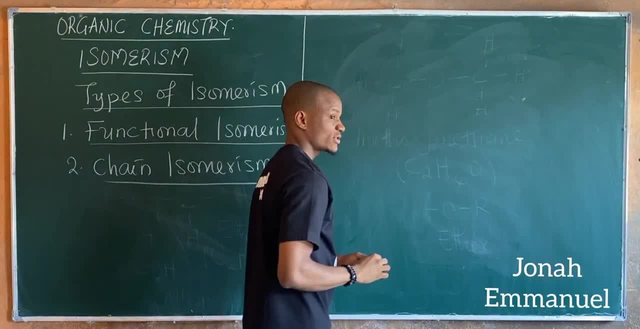 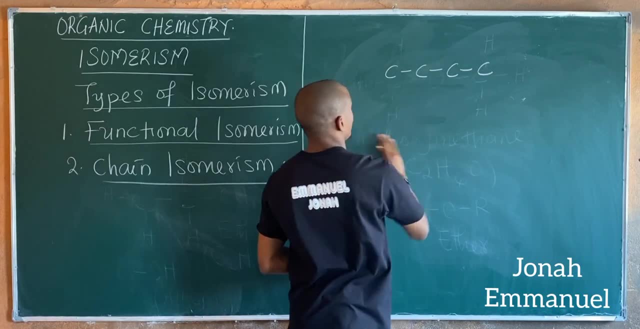 Let's look at butane, For instance. for a boot I'll have 4 carbon atoms, So this becomes 1,, 2,, 3, and 4.. Make this an alkane. This is 1,, 2,, 3,. 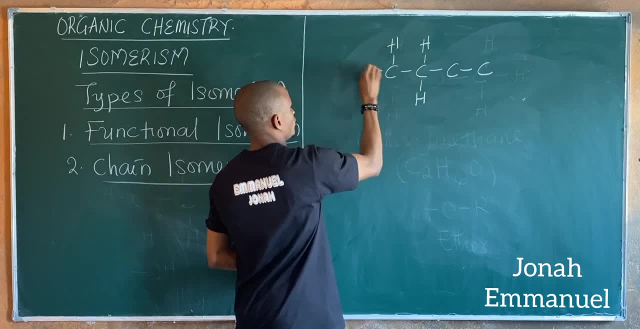 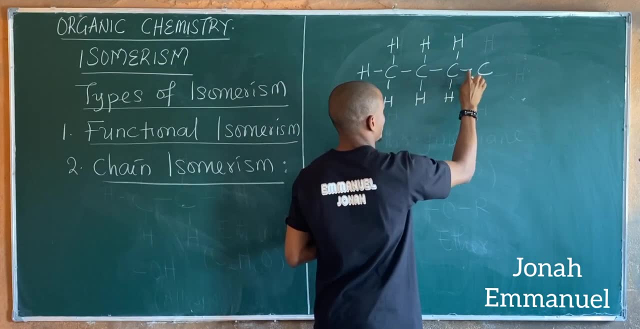 and 4.. This one is 1,, 2,, 3, and 4.. This is 1,, 1,, 2,, 3, and 4.. Here is 1,, 2,, 3, and 4.. So this is my. 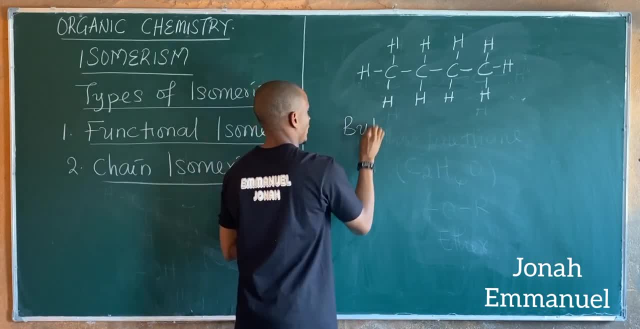 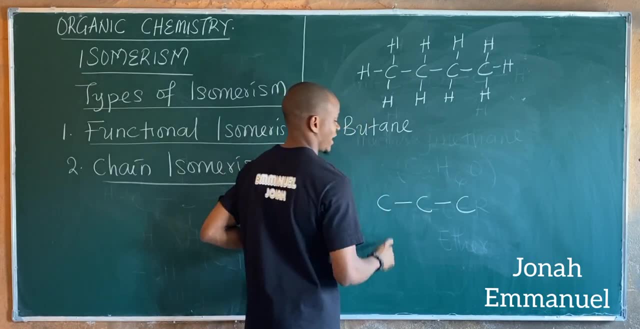 butane atom. This is butane. This is butane. Next up, get 2-methyl propane. For a propane, I'm having 3 atoms, 3 carbon atoms. For 2-methyl it means that the methyl group 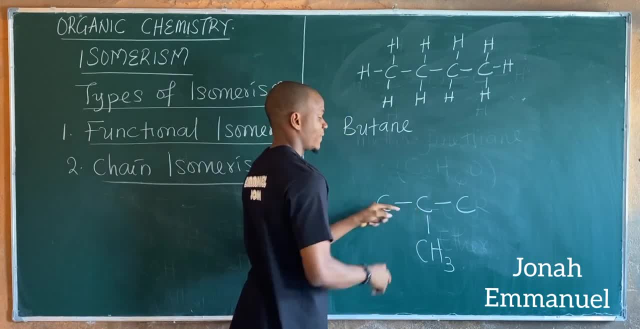 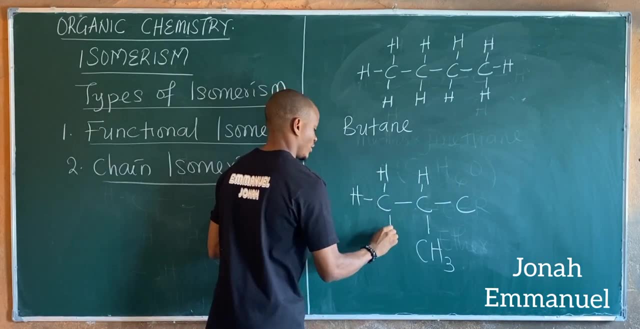 that's CH3 is attached to carbon 2.. Balance this out. This is having 1,, 2,, 3,, 4.. This one is having 1,, 2,, 3, and 4.. 1, 2,. 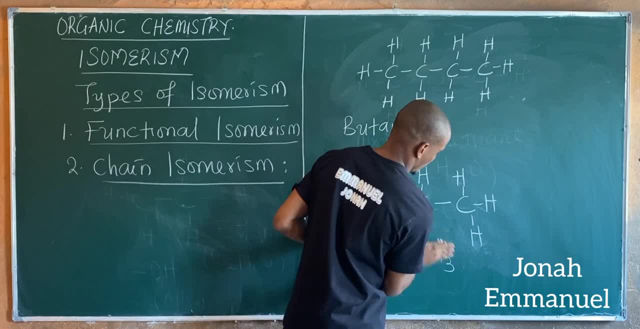 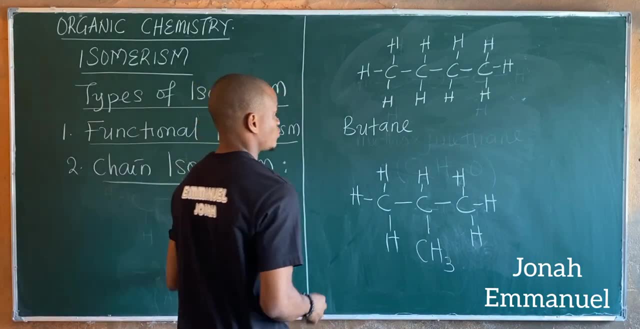 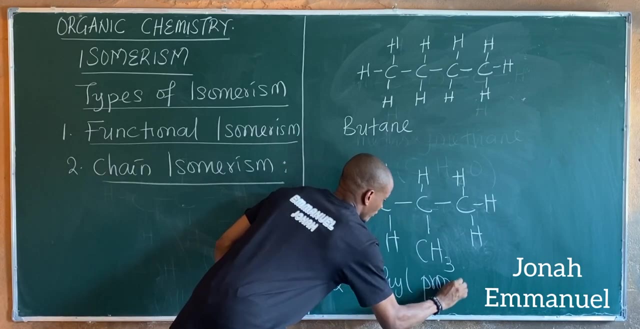 3, and 4.. So I'm having this for my 2-methyl propane. Alright, Count to the number. This is 2-methyl, 2-methyl propane. Combine these two like this. That's more like it. 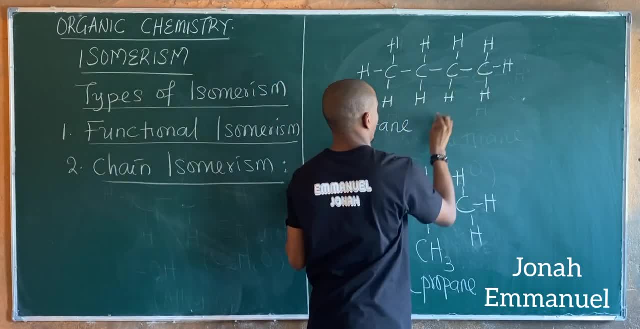 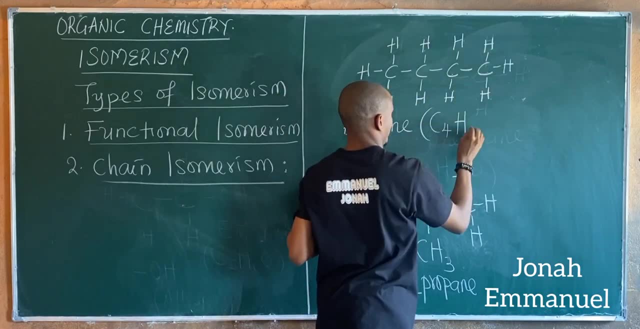 So count to the number of carbon. here I'm having 1,, 2,, 3,, 4.. This is C4.. Count hydrogen: 1, 2,, 3,, 4,, 5,, 6,, 7,, 8,, 9,, 10.. 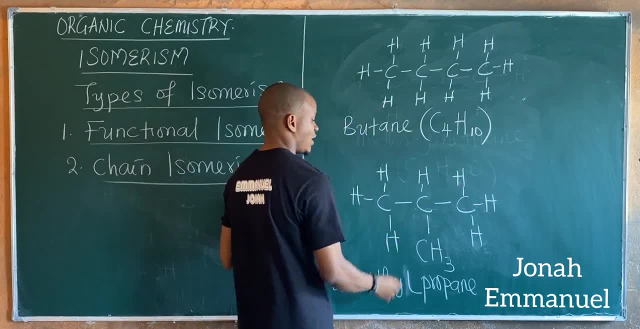 I have 10 hydrogen atoms. For this, count to the number of carbon here: 1,, 2,, 3,, 4.. This is C4.. Count to the number of hydrogen: 1,, 2,, 3,. 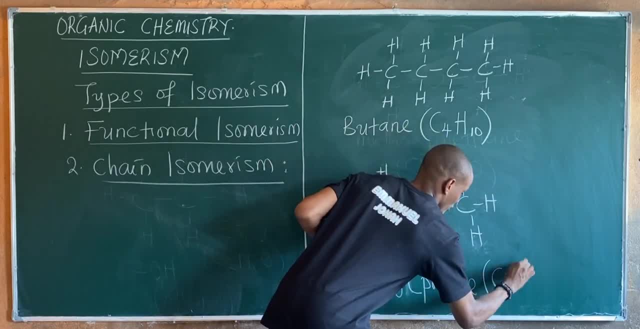 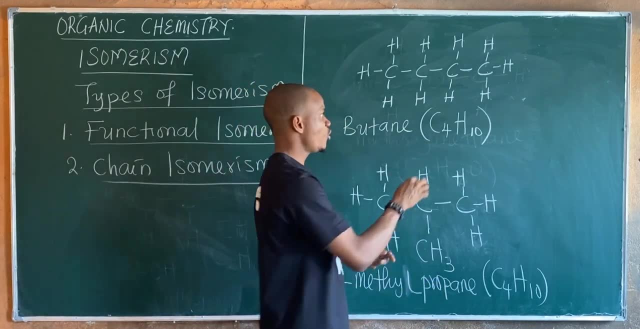 3,, 6,, 7,, 8,, 9,, 10.. I'm having H10.. So we have the same molecular formula, C4H10.. Let's look at the functional group, Obviously for this one here. 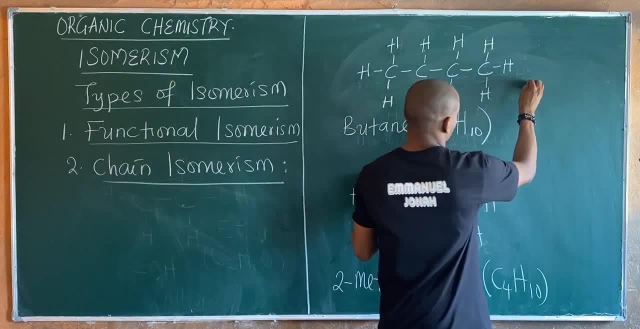 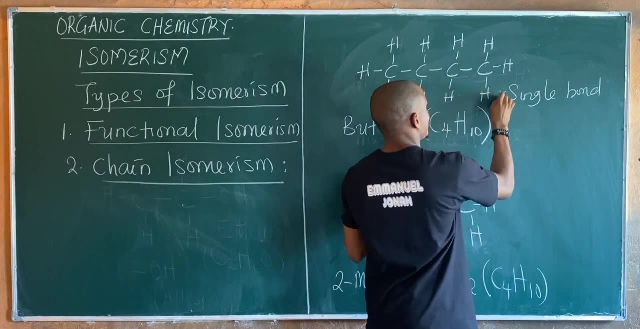 let's look at the functional group. Obviously, for this one here, this is a single bond. for butane I have single bond. That's the functional group. That means it's an alkane For these two. if you look at this structure. 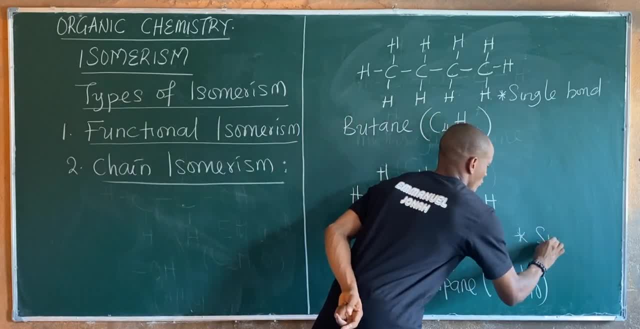 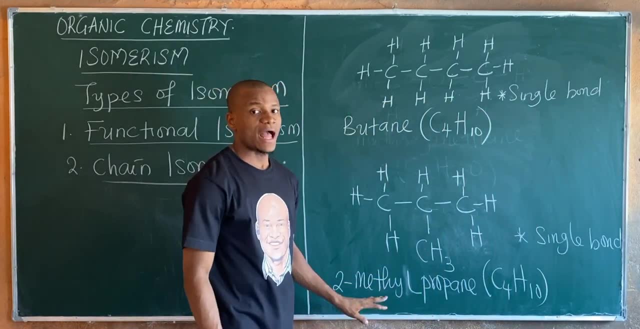 this is a single bond drug, So this one too is also single bond. That means it's an alkane. So both butane and 2-methylpropane are both alkane, since they have single bond. So for these two compounds, 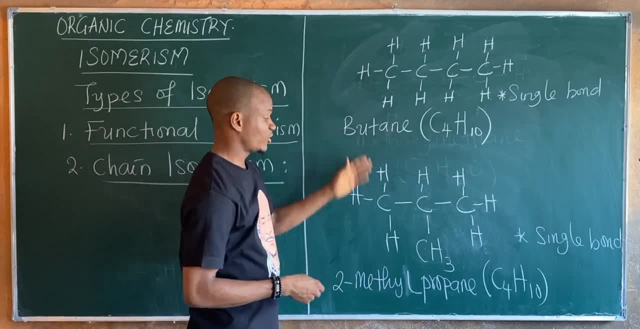 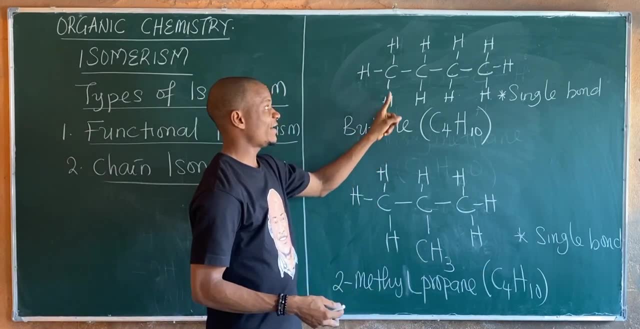 they have the same molecular formula, but different. They have the same molecular formula, They have the same functional group. What's the difference? The difference is in the arrangement For butane. I have the carbon being arranged in a straight file like this, such that 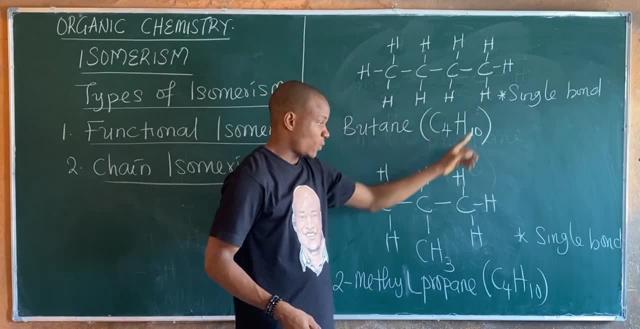 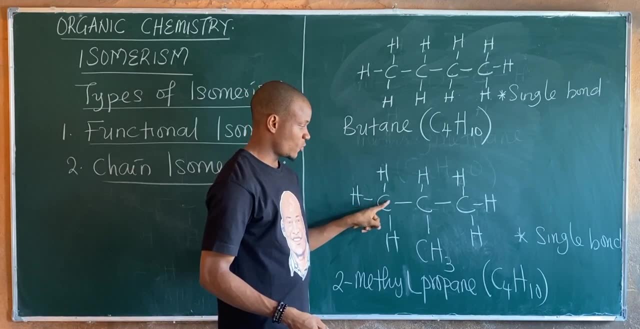 all the carbon atoms are linked to each other, While for 2-methylpropane, the arrangement is that 2-methylpropane is linked to each other. Only three links to each other like this, alright, So only three links directly. This one. 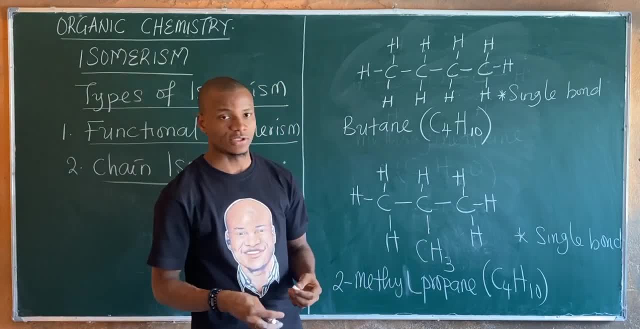 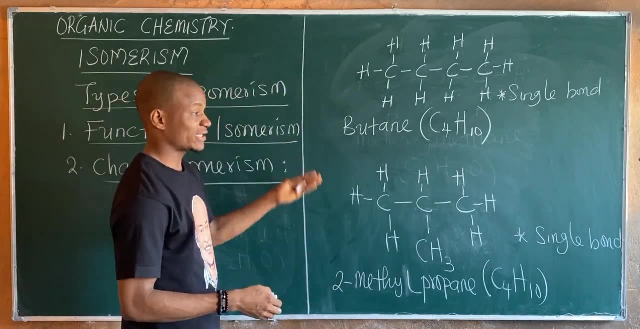 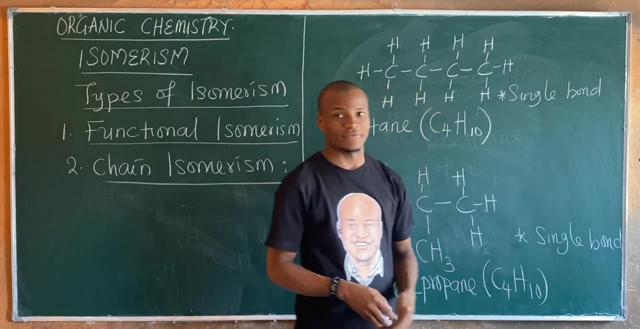 is outside the connection of the carbon atoms. So that's why it's a chain isomerism. That's why they are chain isomers. They are chain isomers because they have the same molecular formula, the same functional group, but different. 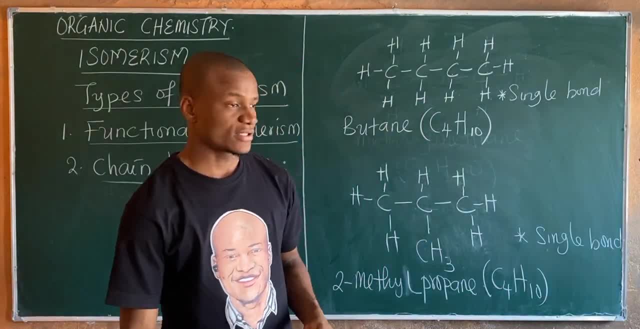 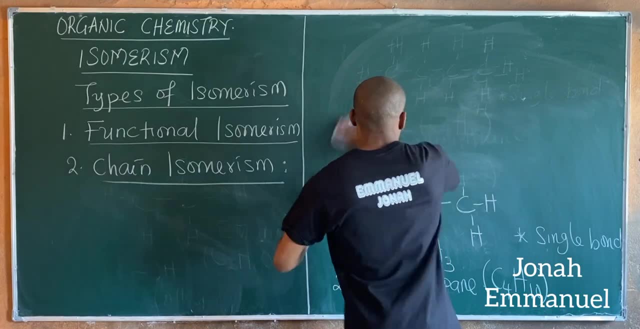 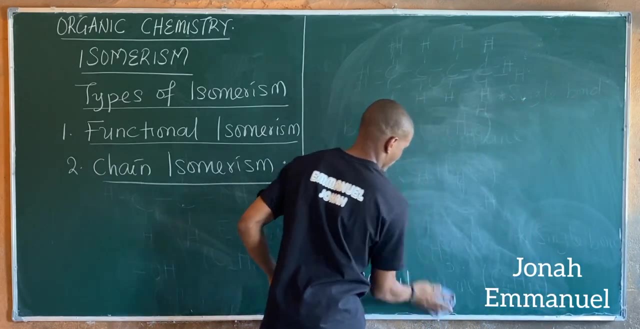 arrangement of the atoms in space. So this is a second type of isomers of the apps, Second type of isomerism that exists. Look at the third and final type of isomerism that we can get, The third type of isomers or isomerism. 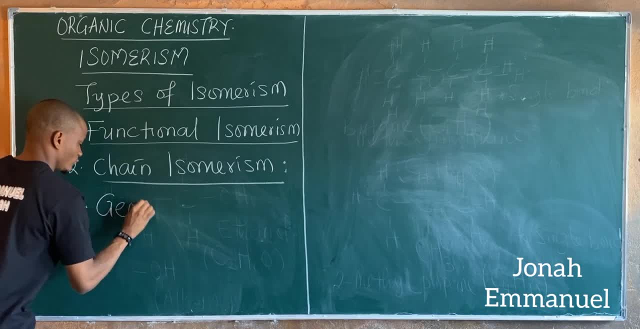 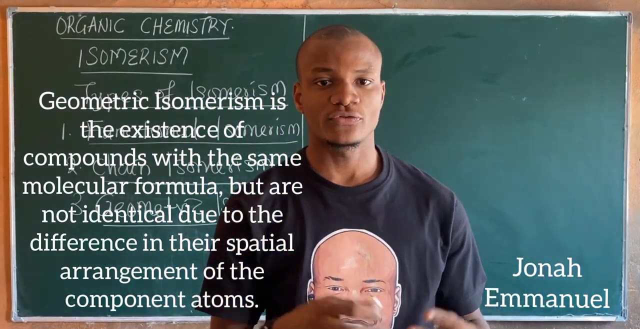 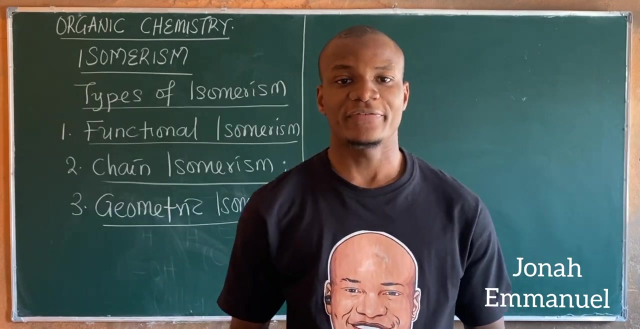 that exists is known as geometric isomerism. Geometric isomerism is the existence of two or more hydrocarbons with the same molecular formula but are not identical due to the difference in the spatial arrangement of the component atom. When it comes to geometric isomerism, or geometric isomers. there are two types of geometric isomers. The first one is known as the cis and the second one is known as the trans. So you have cis, trans and trans type of geometric isomers. Alright, so I'll take some examples. 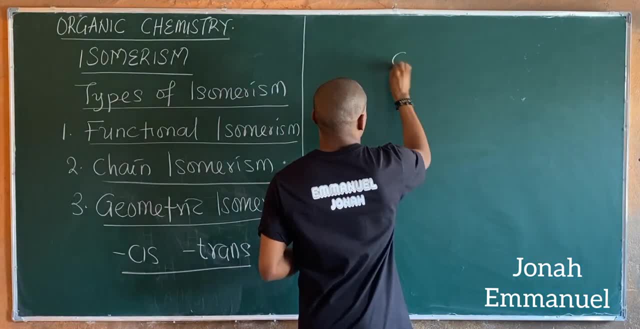 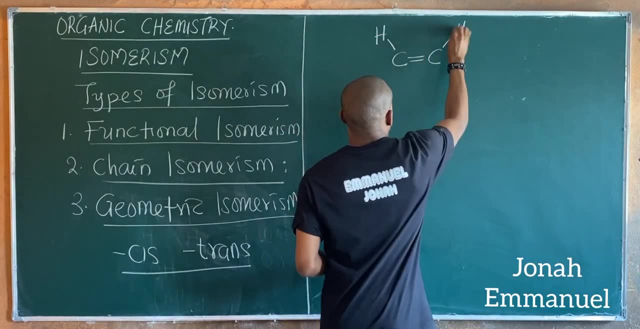 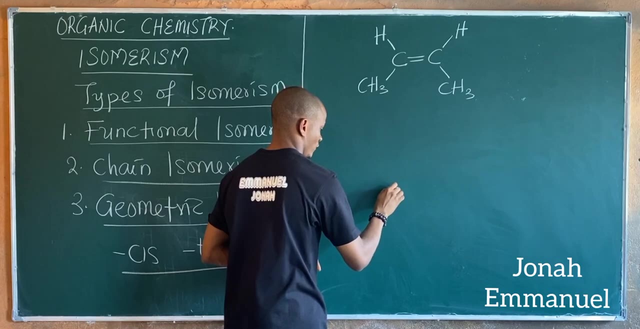 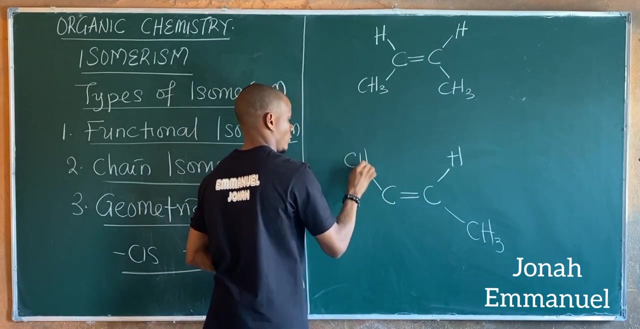 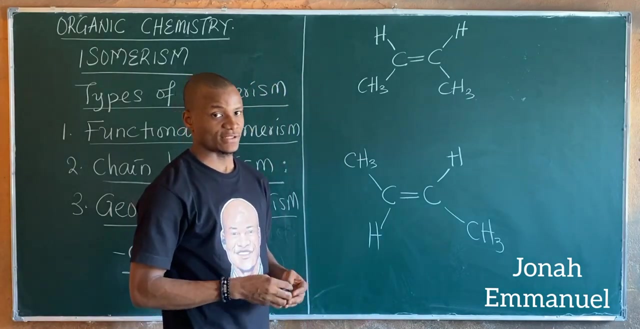 and illustrate this. If I have a compound such as this, something of this nature, Alright, and I have a compound also of this nature. Now, if you look at this and this, they are almost alike, but there are some differences or there's a difference, The major difference between 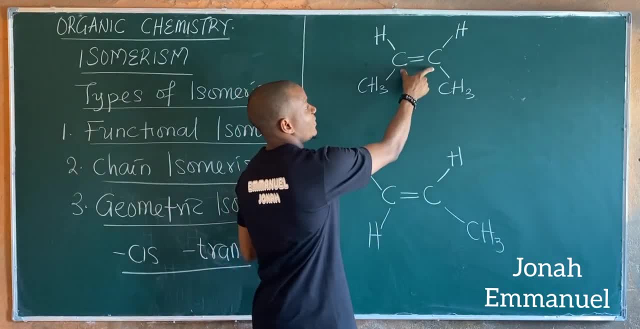 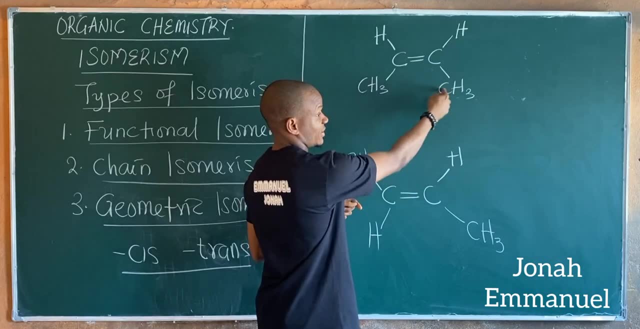 this compound here and this one is that for this particular compound here, the alkyde group, that's this, and this being metal, the alkyde group, are like in the same plane. So you can see here why for this, for this particular compound here, 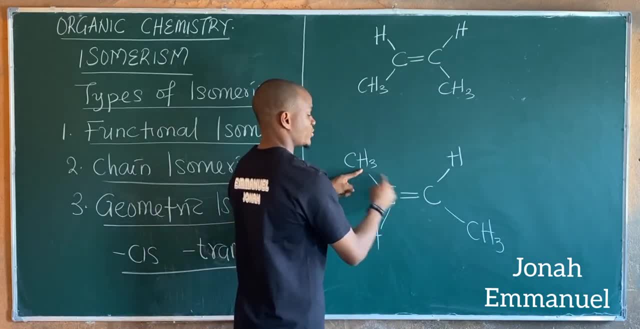 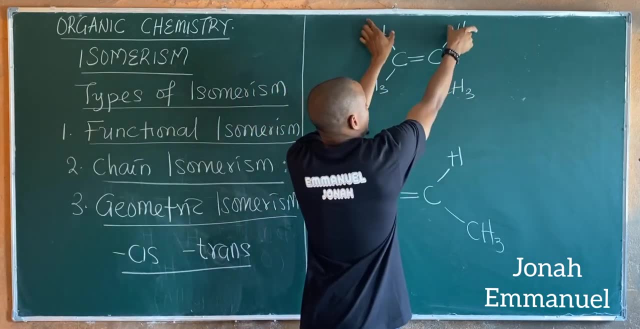 the alkyde group are like opposite to each other. Alright, so when you have a case where the alkyde group are in the same plane, whether downwards or upwards- in this case, what you have here is a cis. This is known as cis. 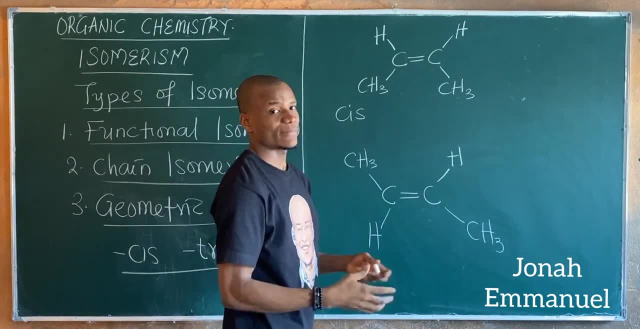 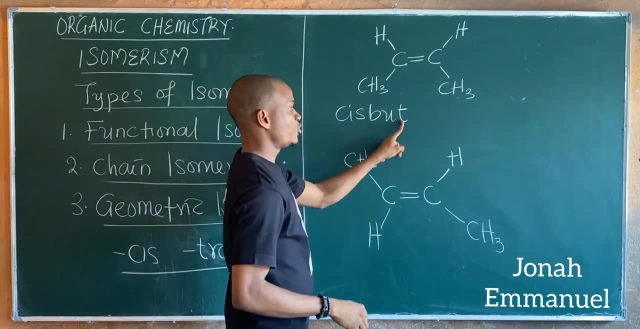 Cis, what Count longest continuous carbon chain? This is 1,, 2,, 3,, 4.. 4 is boot. So we count cis, boot, Boot, because I have 4 carbon atoms. Next up I will count from. 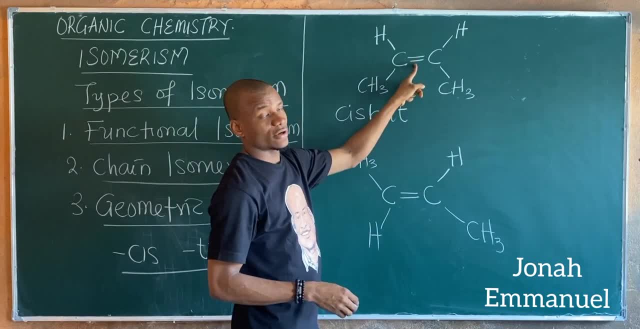 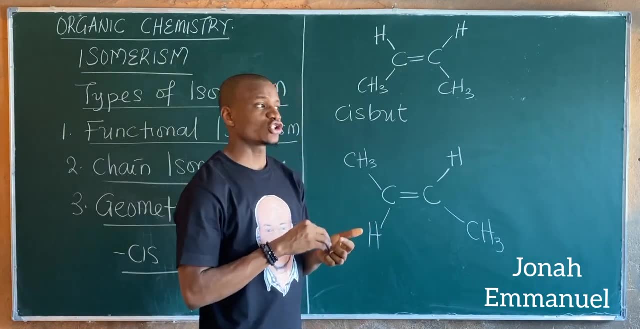 this way here. Usually this is an alkene, Alright, Alkene because it has double bond. Usually, when it comes to alkene, it's necessary that you show the position of the double bond in your naming. Alright, If I count. 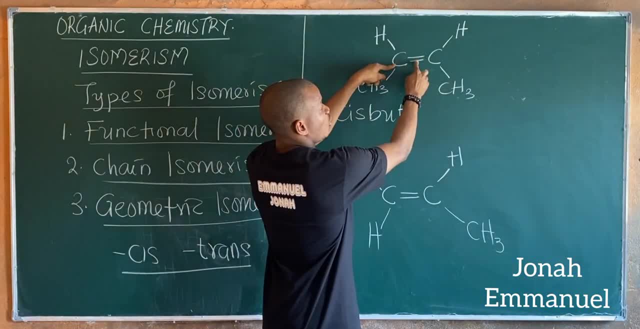 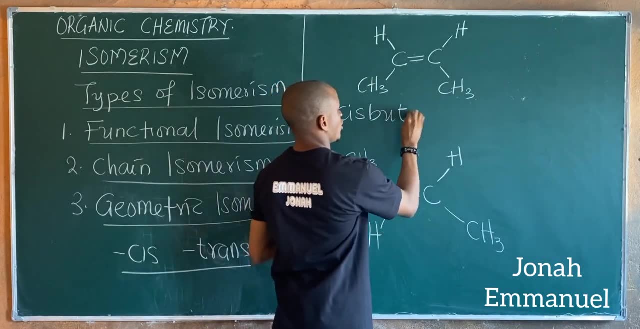 this way, this is carbon 1, 2.. Hence double bond occurs at carbon 2.. If I count this way, this is 1, 2.. Hence double bond occurs at carbon 2.. So this becomes cis boot 2. 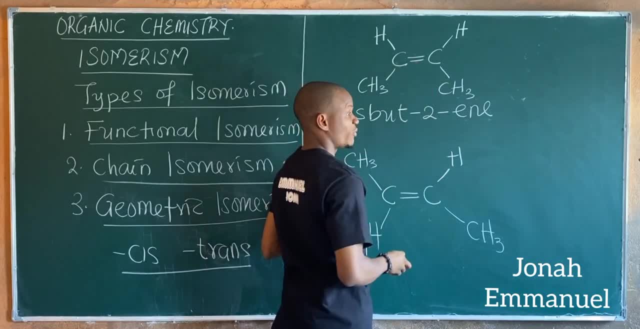 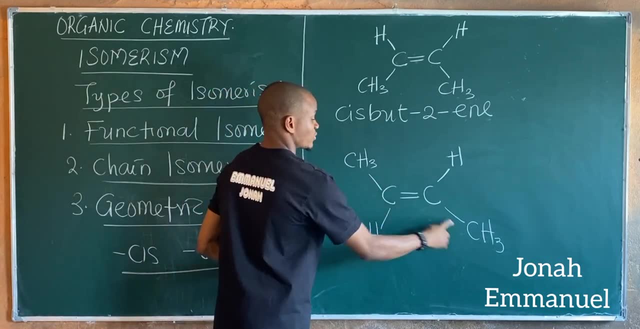 and then in: In, because it has double bond in and alkene, So the in is for alkene. In this case, here, when the substrates are in opposite positions, it's called a trans. So this is called a trans. 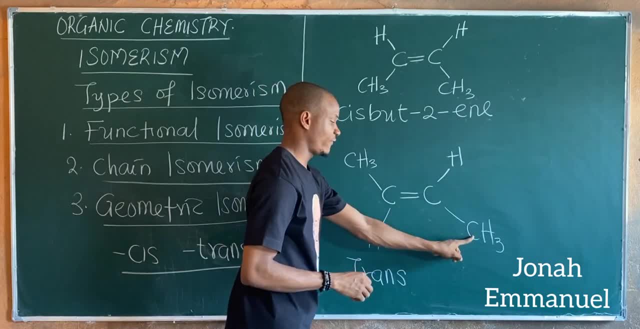 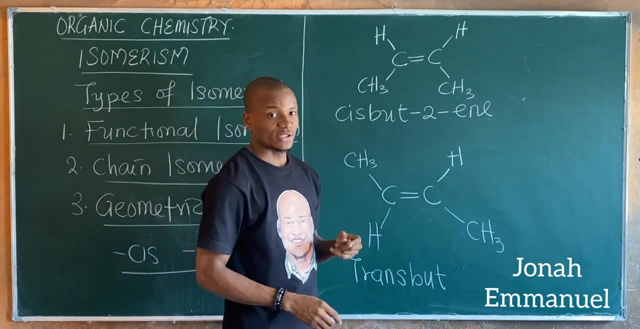 Count the total number of carbon atoms: 1,, 2,, 3,, 4.. So it becomes 4.. It's a boot, So it becomes trans boot. Locate the position of the double bond. This is 1, 2.. 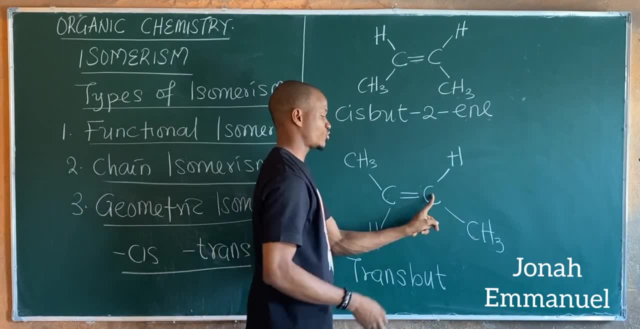 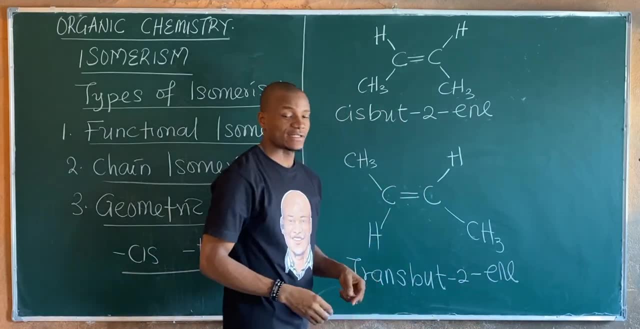 Double bond is at carbon 2.. Locate this way I'm having 1, 2. Double bond is at carbon 2. So it becomes trans boot 2 in In because it has a double bond. So this is the technique of. 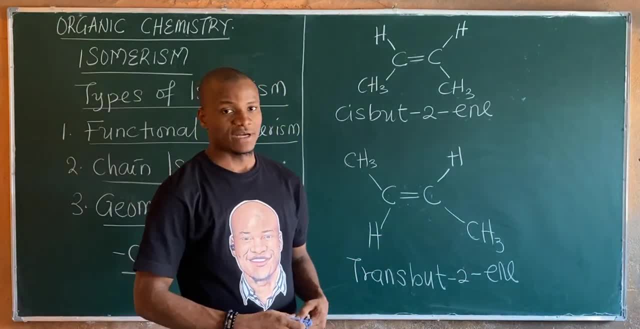 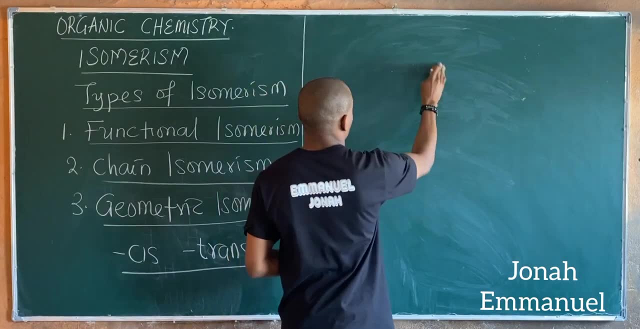 naming geometric isomers. We'll take one more example and we're done with this Geometric isomerism, and then we'll end with this: Alright, let's say I have compounds such as this: Carbon double bonded to carbon used in a hybrid. Let's say: 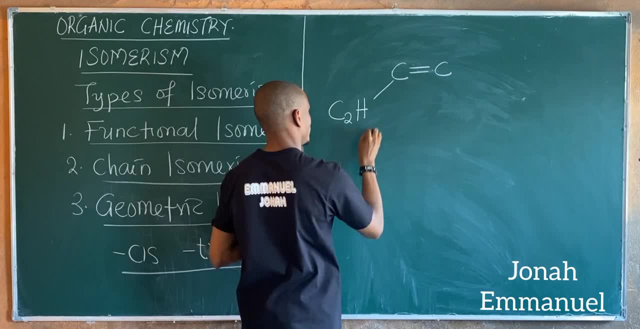 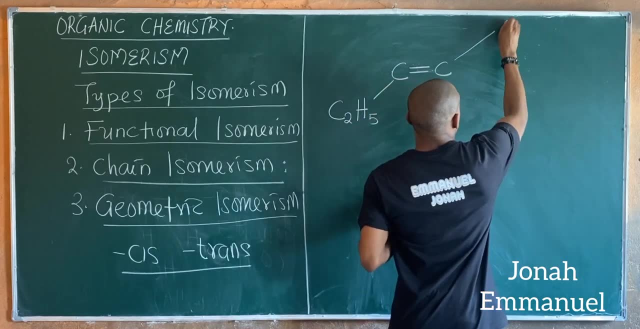 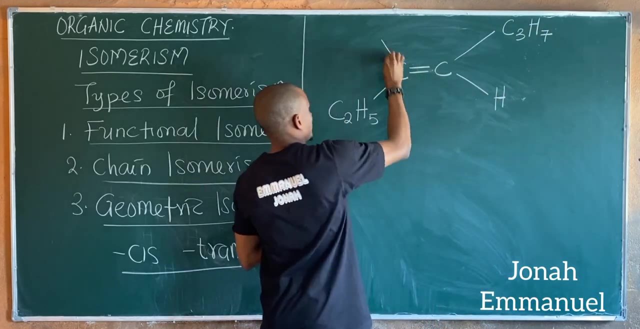 this time at zil. Okay, I have this one here. Okay, So I use propyl, for instance. Then bring hydrogen this way, and then bring hydrogen this way. Let's say, I have something up in here, This this way. 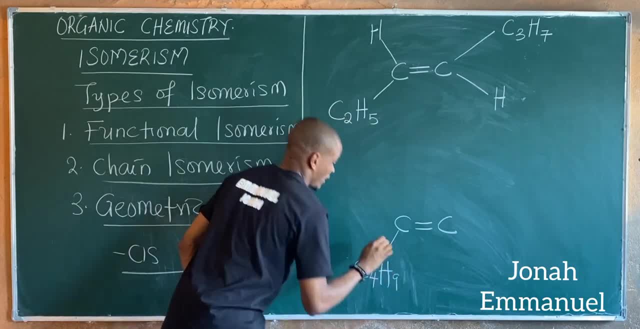 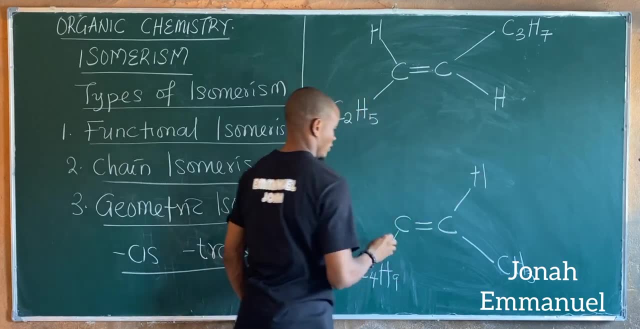 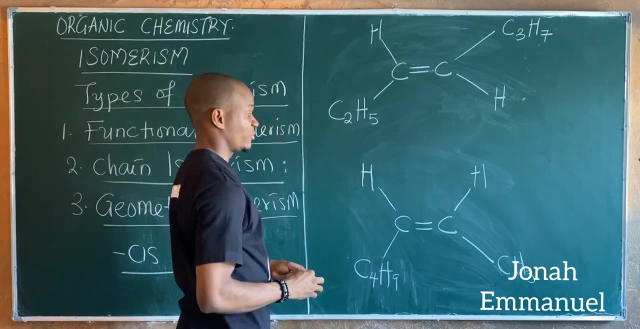 Call this C4H9.. That's propyl, This one here, CH3.. That's metil. Let's try to name these two geometric isomers Or these compounds that exhibit geometric isomerism. This one is not exactly isomers, though. 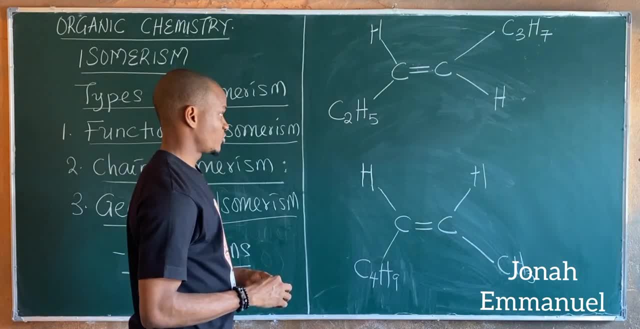 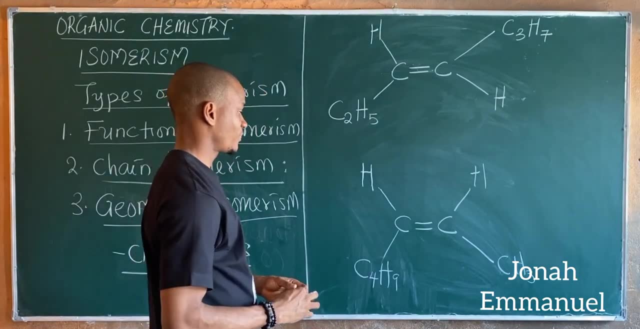 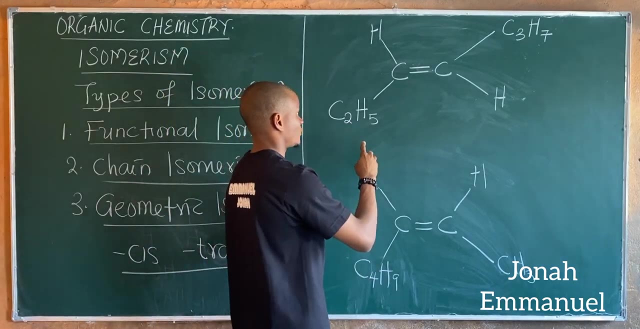 They're not exactly the same kind of isomers, though, But we're just trying to see if we can. Okay, Yeah, So let's try to name this compound For this. now I'm having case 1.. This is a trans system. 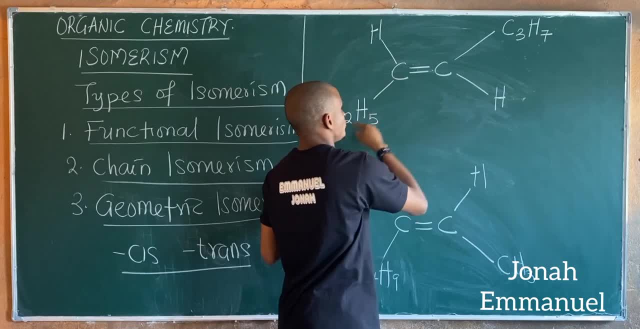 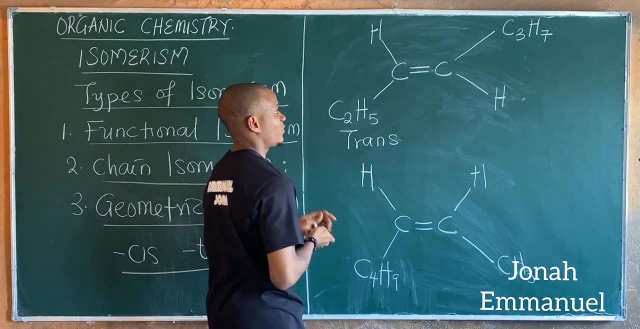 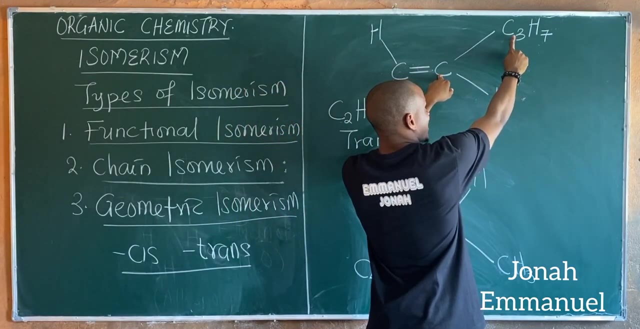 I alsoery in here. It's trans because they are actually opposite each other. That becomes trans Trans. Next up get contact about carbon atoms. Two carbon atoms here. This is 2, 3, 4.. 4 plus 3 here.